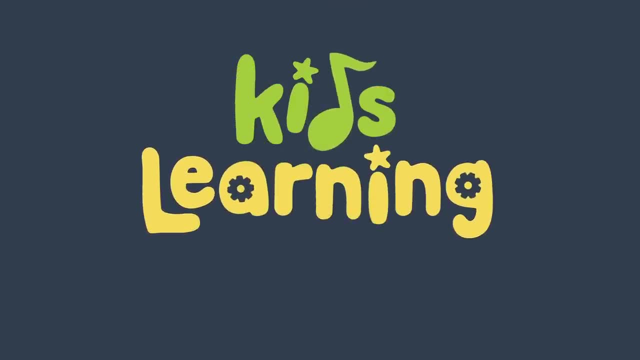 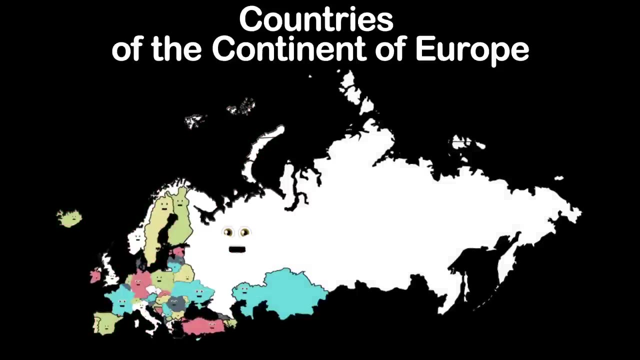 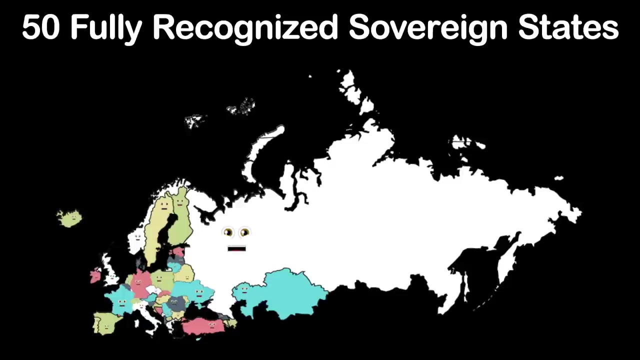 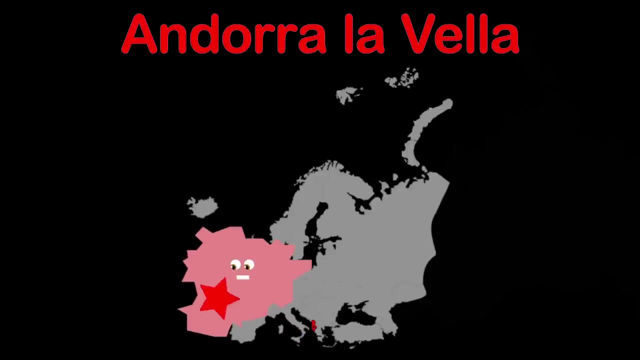 We are the countries of the continent of Europe, the northwestern portion of the larger landmass called Eurasia. We're the countries of the continent of Europe, 50 fully recognized sovereign states that we will teach you. I am Albania, this is Tirana. I'm Andorra- this is Andorra. 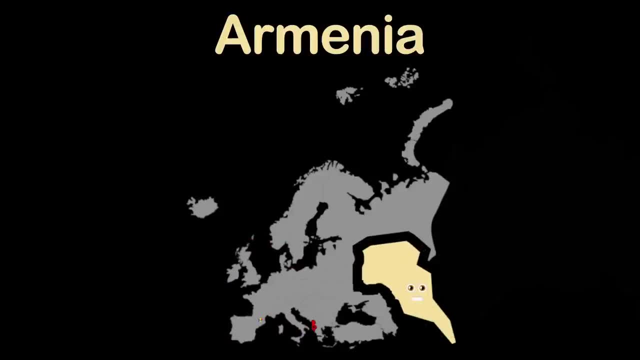 la Bella. Armenia's in Europe and Asia, and this is Yervon. My name's Austria, my Vienna has so much charm. Azerbaijan's in Europe and Asia, and this is Baku. My name is Belarus, and Minsk is right here, it's true. Belgium here, and this is Brussels, you see. 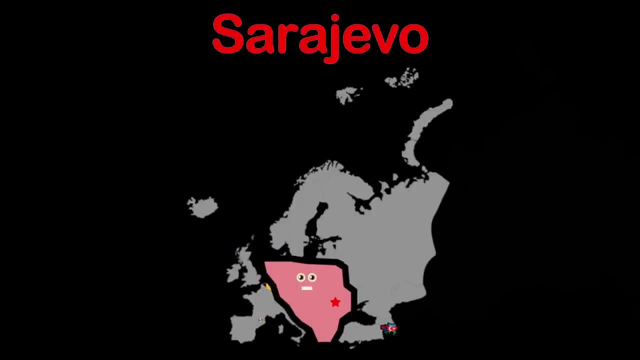 Bosnia and Herzegovina. Sarajevo is in me, I'm Bulgaria and this is Sofia. I'm Croatia, my capital's, Zagreb, you saw, And I am Cyprus. this is Nicosia, Czech Republic's, here in Prague. guess what you just saw? My name is Denmark and Copenhagen is here Estonia's. 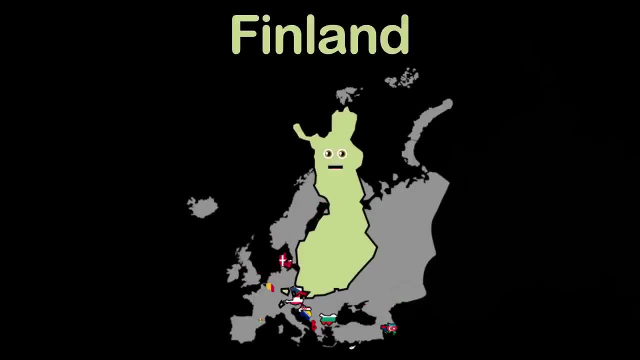 here and Tallinn just appeared. You're seeing Finland, you're seeing Austria, you're seeing Helsinki is the star. Welcome to France. get to Paris by car. Georgia's in Europe and Asia capital's Tbilisi. My name's Germany, and Berlin is what you see. I am the country. 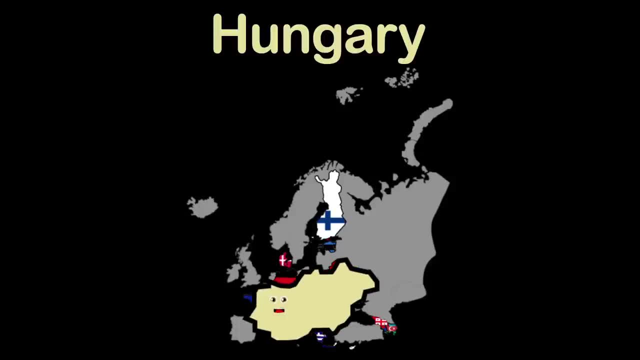 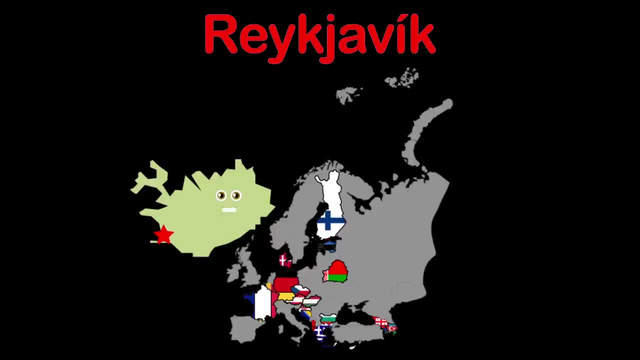 of Greece. Athens is beautiful. My name's Hungary. Budapest is my capital. I am Iceland. Reykjavik is my capital's name. I am Ireland. Dublin's my capital. This is Italy. Rome has fame in history. I'm Kazakhstan in Europe and Asia. Estonia is in me. 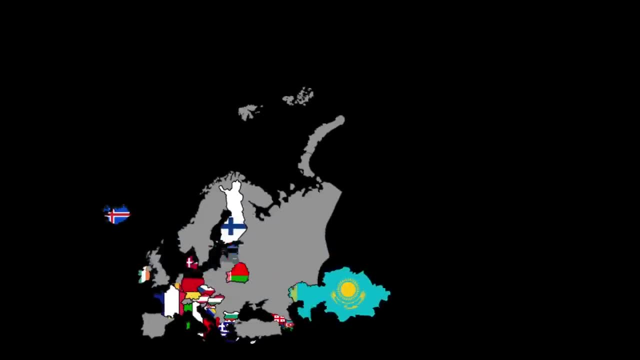 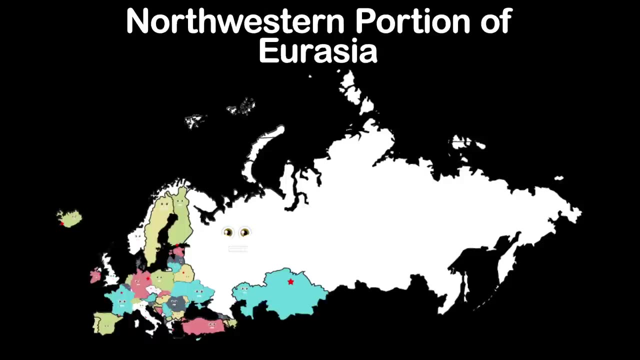 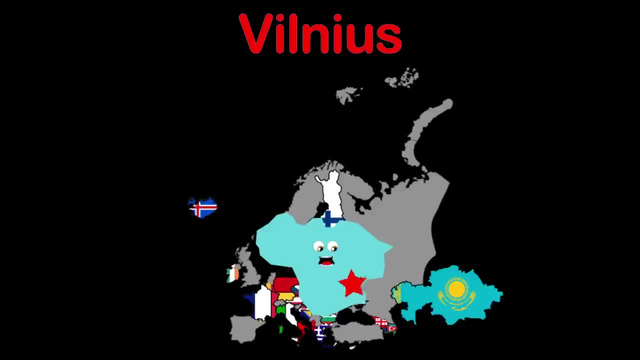 I'm Lithuania. Vilnius, I introduce Luxembourg, is here and this is Luxembourg City. I'm Macedonia and this is Skopje. you see, This is Malta and my capital is lens. You'll just now is what you saw: Monaco. my capital is also called Monaco, Pdies as my. 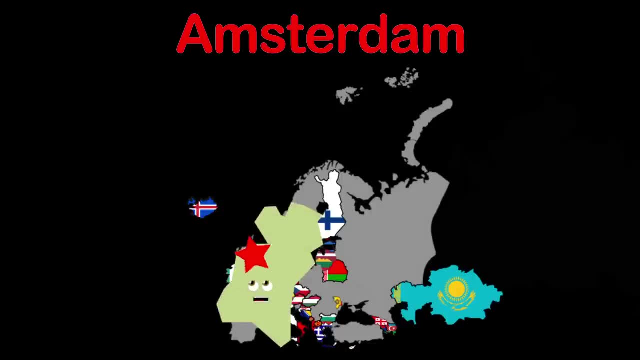 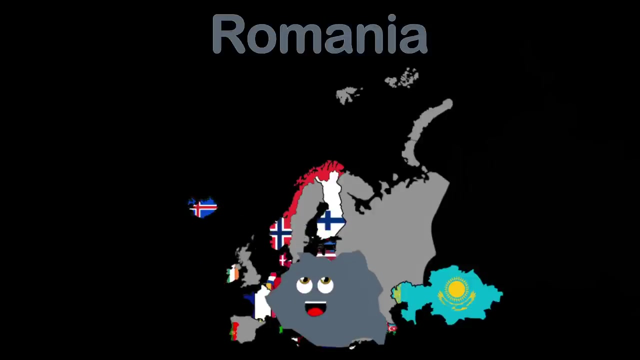 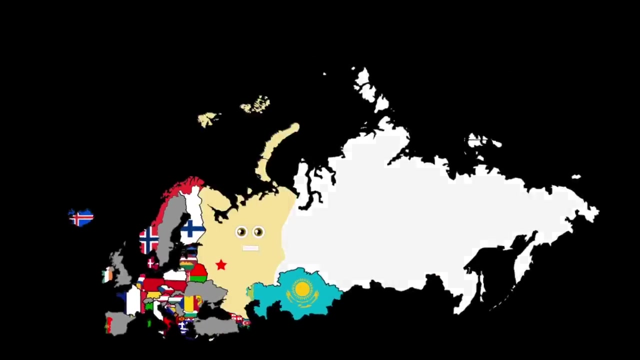 capital. I'm the Netherlands and this is Amsterdam, Norway. here now you're seeing Oslo, man, My name is Poland. My capital's name is Warsaw. I am Portugal. Lisbon is what you just saw. I'm Romania. This star is Bucharest, Russia's in Europe and Asia, Moscow is the best. This is San Marino. San Marino is a. 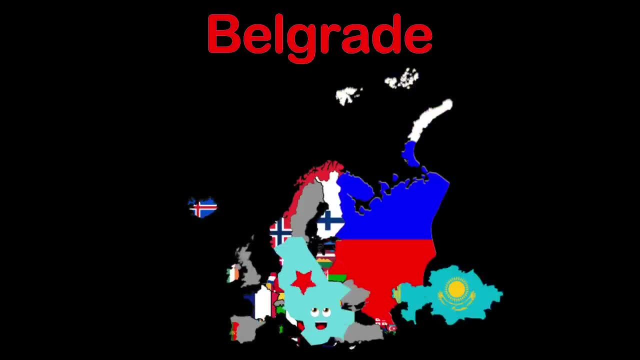 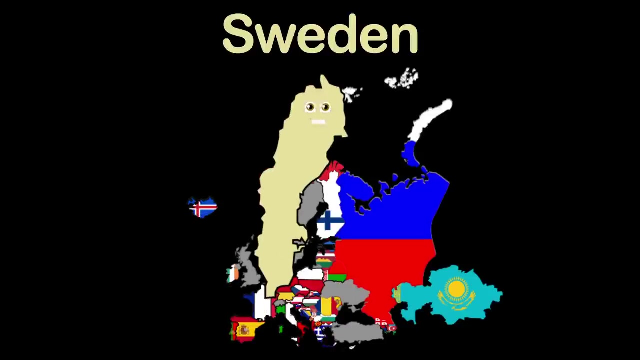 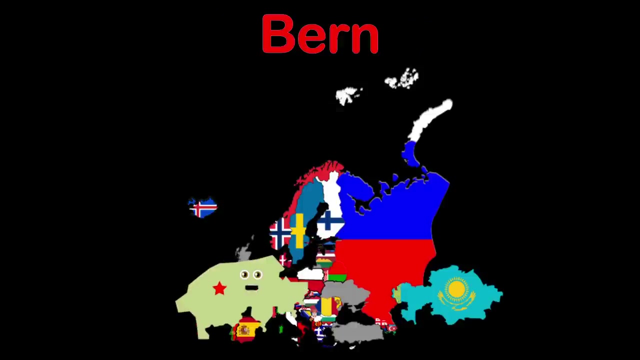 wonderful place. I'm Serbia and my capital's Belgrade. Slovakia, here, and this is Bratislava. I'm Slovenia and this is my capital, Ljubljana. My name is Spain and this is Madrid. Sweden is here, Stockholm's where this star sits. I am Switzerland and my capital's name Bern, Turkey's in Europe, and 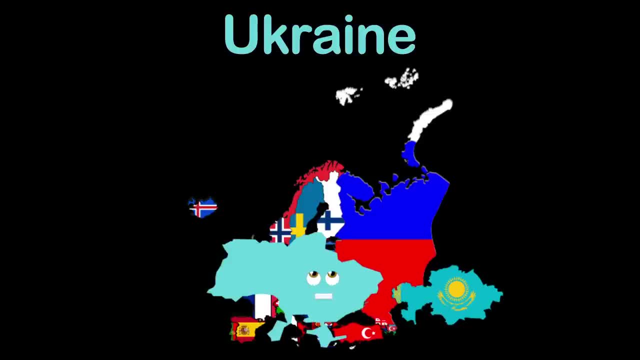 Asia, Ankara's where this star turns. Sweden is here and this is my capital, Kiev. I'm the United Kingdom, or UK London's a name. I just said Vatican City or Holy See. Vatican City is the capital that resides in me. We are the countries. 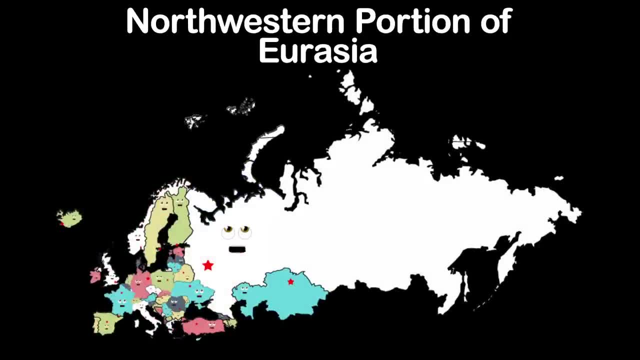 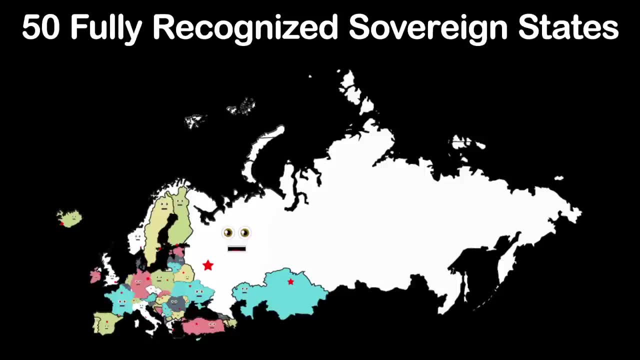 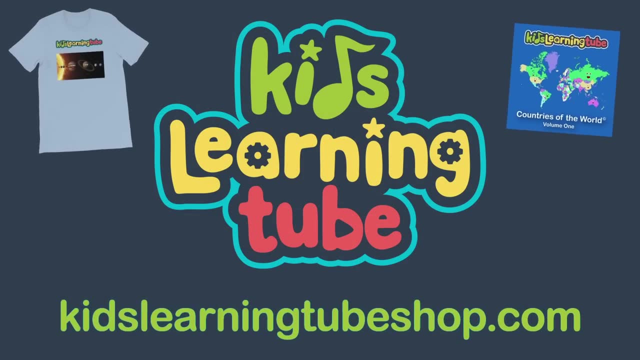 of the continent of Europe, The northwestern portion of the larger landmass called Eurasia. We're the countries of the continent of Europe: 50 fully recognized sovereign states that we will reach up. Get your favorite Kids Learning Tube t-shirt or song today at kidslearningtubeshopcom. And don't forget to subscribe Kids Learning Tube. 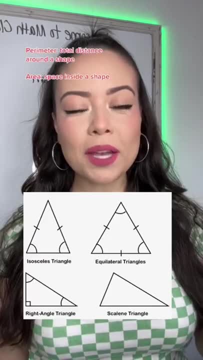 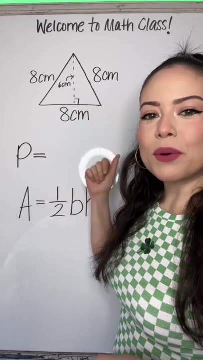 Let's talk about area and perimeter of a triangle. Perimeter of any triangle can be found by adding all three sides versus area can be found by using the formula 1 half base times height. Let's look at this triangle, for example. If you notice, we actually have an equilateral triangle.